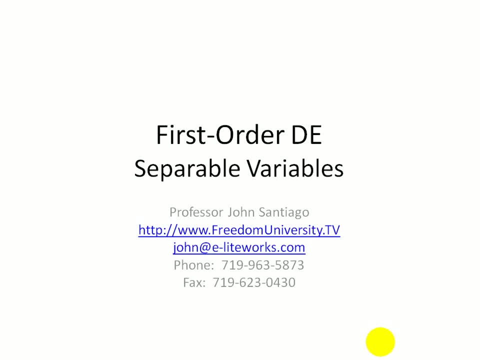 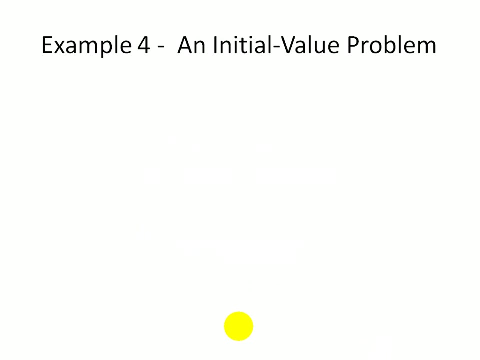 We're going to continue our discussion with force order differential equations using the method of separable variables, and we're going to apply this concept, this method, to an initial value problem. Here's another example of an initial value problem. You're going to have to recall some trigonometric identities, as well as integration by parts. 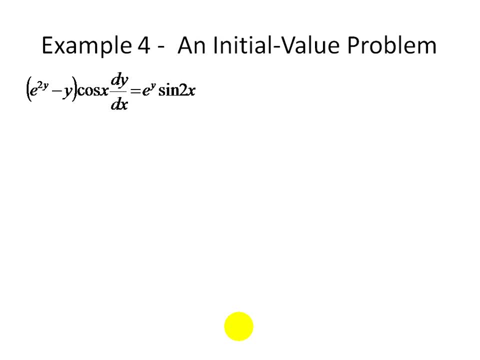 So let's say we're given this expression e to the 2y minus y. take that quantity, multiply it by cosine x and then multiply it by dy. dx is equal to e to the y sine of 2x. We have an initial value: y0 equals to 0. That's our initial condition or initial value. 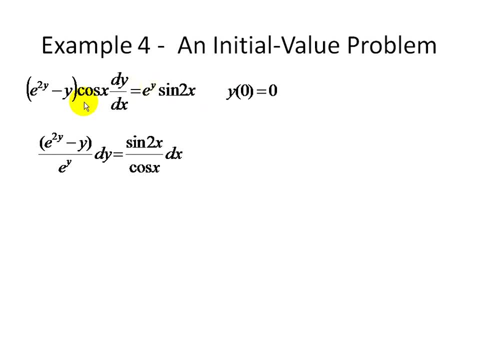 Next we divide cosine of x on both sides of this equation, So that leaves e to the 2y minus y. divided by ey, dy is equal to sine of 2x, cosine of x, dx. Again, we're using the method of separable variables, where we isolate on one side a single variable, in this case y. 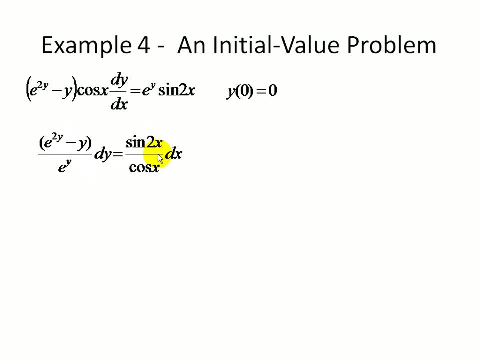 and on the other side a single variable- in this case y- And on the other side a single variable- in this case y- And on the other side we isolate into another single variable, and in this case it's x. Now we can simplify: on the right-hand side: e to the 2y divided by ey leaves ey. 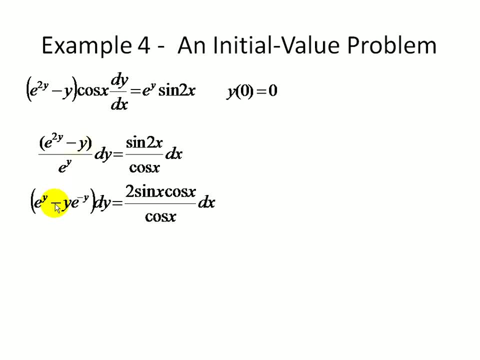 and then negative y over ey leaves negative y e to the minus y dy. There's a trig identity sine of 2x and we can express it alternatively as 2, sine x times cosine of x. Well, we see, this cosine of x cancels out this cosine of x, so this leaves sine of x multiplied by 2.. 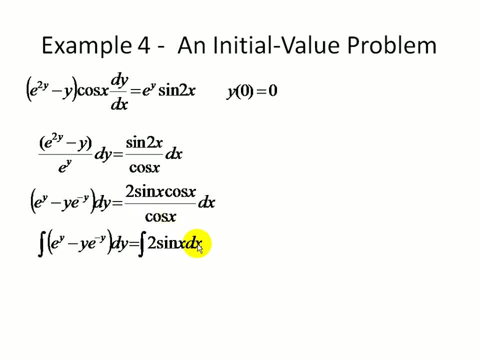 So this is what's left on the right side of this equation and we're going to integrate both sides of this equation now. So here, we'll integrate this later, But we'll focus now on the left side. We're going to do the integration by parts. 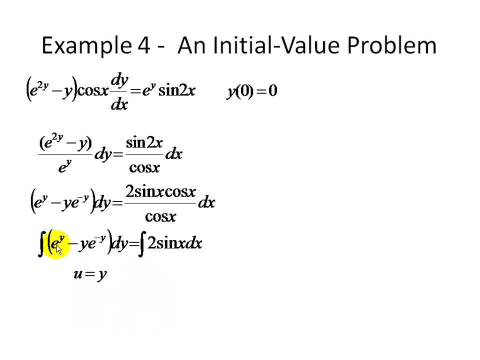 So this is the first term here- is easy to integrate. It's just simply e to the y, And so the integration of part will occur here. Now you define: u is equal to y, dv will be e to the minus y, dy, and that's expressed here and we'll put a minus sign. 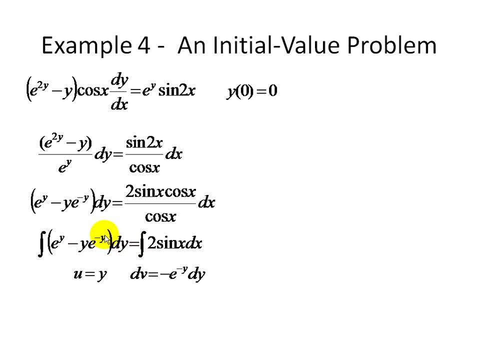 So that's your u dv And that's your v integral. when you substitute it right here, Now v, we take this expression and we integrate: this is just simply e to the minus y, And then taking the differential on both sides of this equation yields du equal to dy. 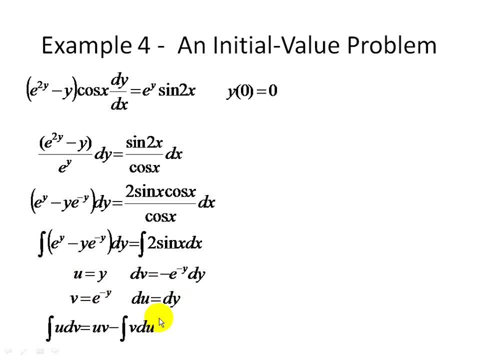 Now we do all this substitution that we defined here and substitute it in this expression. Now we know that we're going to integrate this, and we're going to integrate this and we're going to integrate this. Note that u dv is once again this expression here. 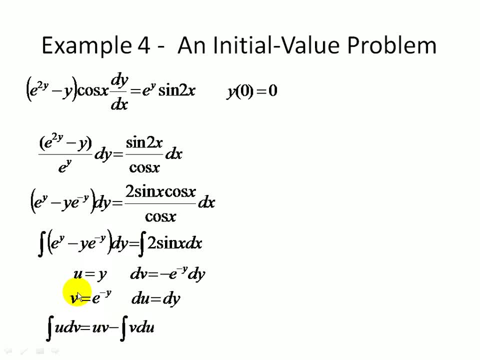 And that uv is defined here, Here's u and here's v. We're going to subtract this with this integral v, which is e, to the minus y, du, which is simpler to integrate. When we do that we have, for the first term is just ey. 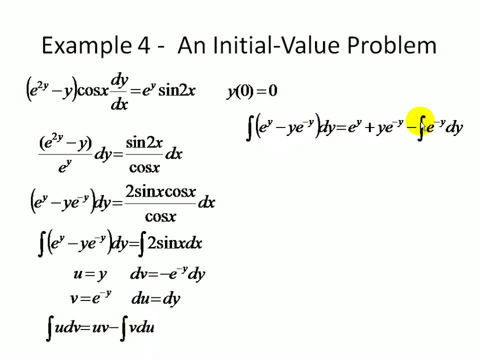 And then this term, This term right here, consists of these two terms. Now, this is the uv term, u against this y, and v is e to the minus y. So that's what this first term is. And then this term is a result of substituting for v right here and du for dy. 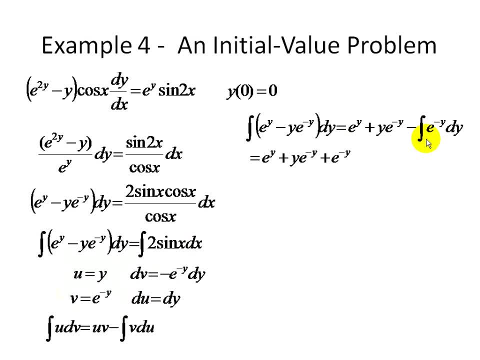 So you can see that this is simpler to integrate. Now, when we do that, we get e to the y plus y, e to the minus y. So that's these terms, And then this term right here is just simply e to the minus y. 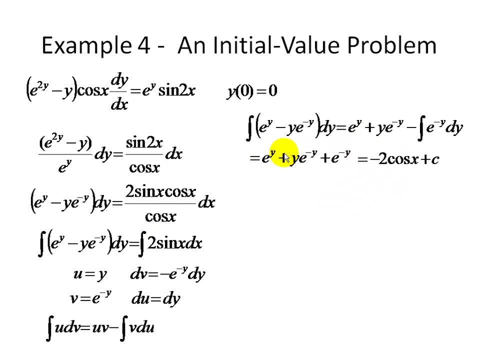 When you integrate the right side- we just completed the left side- Now, integrating the right side, we have that equal to negative 2 times the cosine of x plus c, where c is an arbitrary constant. Now we can get rid of this arbitrary constant by applying our initial value or initial condition.